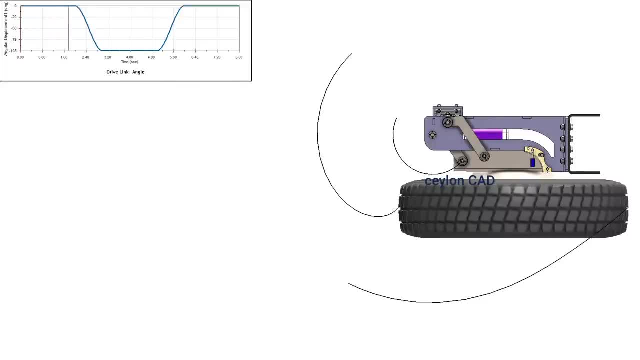 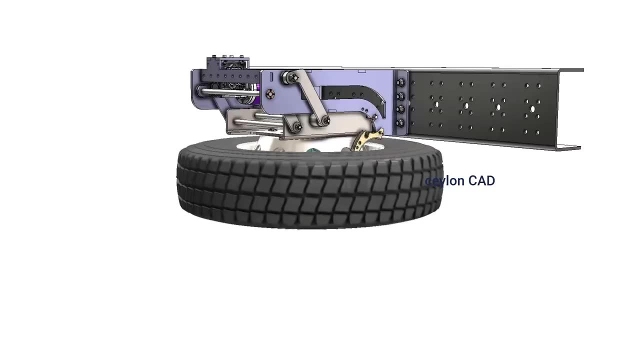 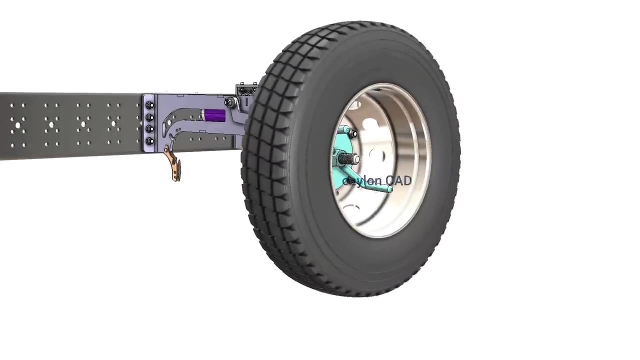 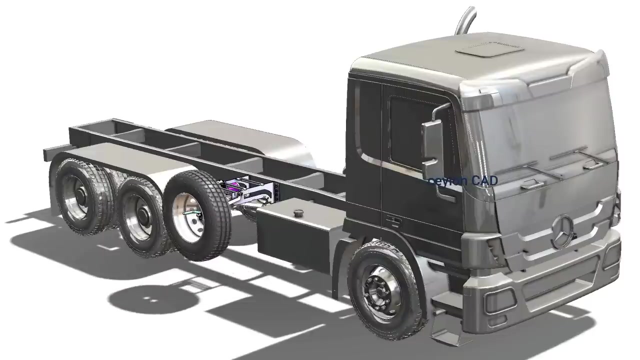 Just treat your body as mine, Baby. you'll get me high and dry. You're giving me wind and rain. You're some kind of butterfly, Baby. you'll whip up my appetite. Baby, you'll get me this night. You'll whip up my appetite. Don't leave me here high and dry. Oh, oh, oh. I don't wanna jinx it, baby, Just not get ahead of my time. Oh, oh, oh, But I don't really miss you, baby. Baby, you'll get me high and dry. Oh, oh, oh, Cause I stand up and speak with my mind. 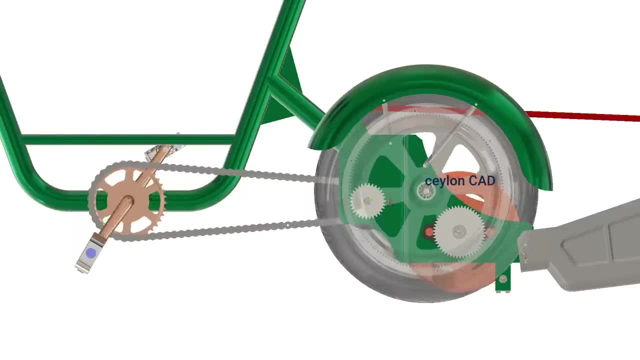 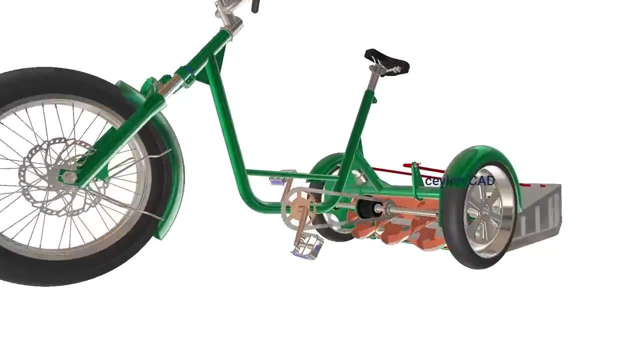 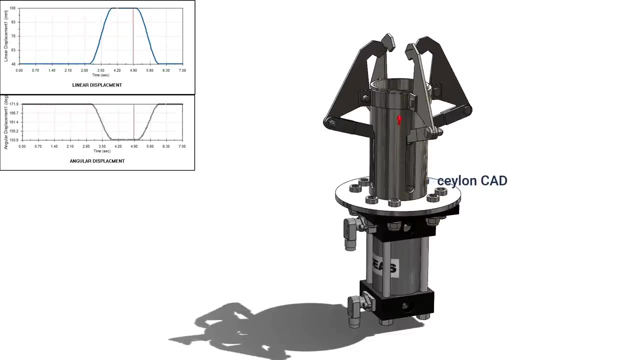 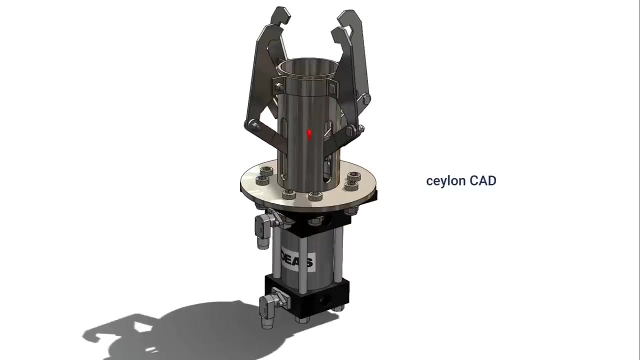 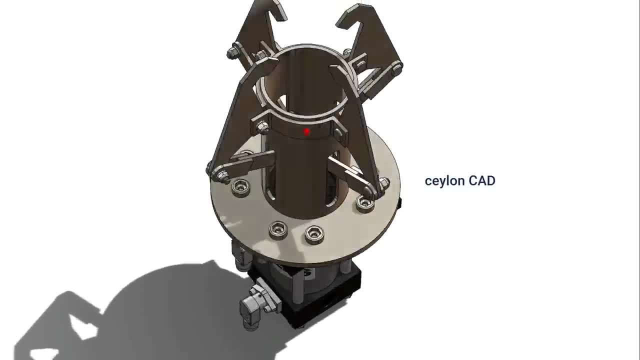 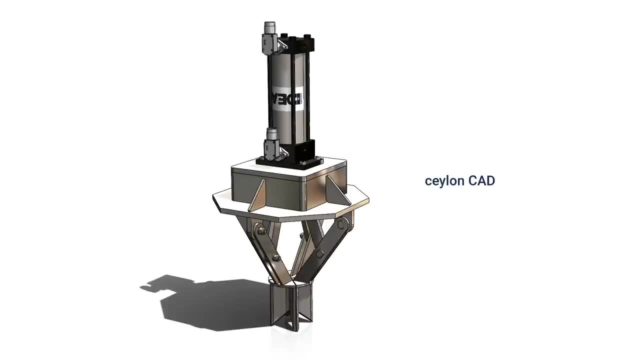 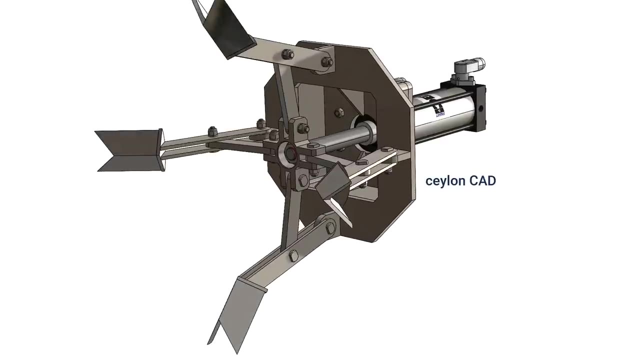 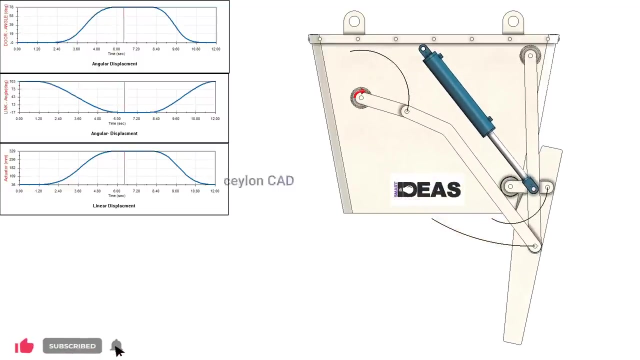 Oh, oh, oh ¶. Baby, you give me ice and fire. ¶ You're chilling in the rain. ¶ You're some kind of butterfly ¶. Baby, you give me good night eyes. ¶ You whip up my appetite ¶. Don't leave me lying dry. ¶. Baby, you give me ice and fire. 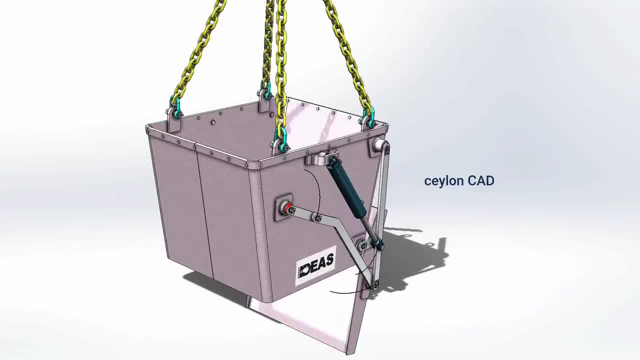 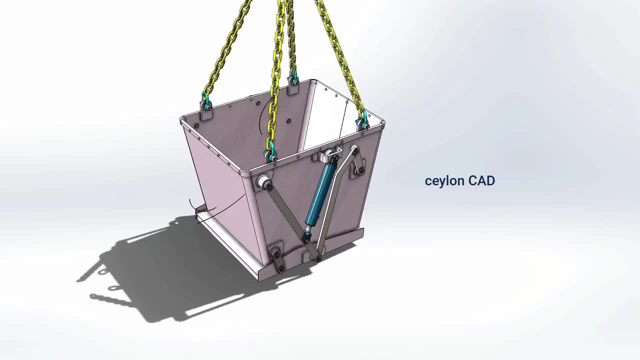 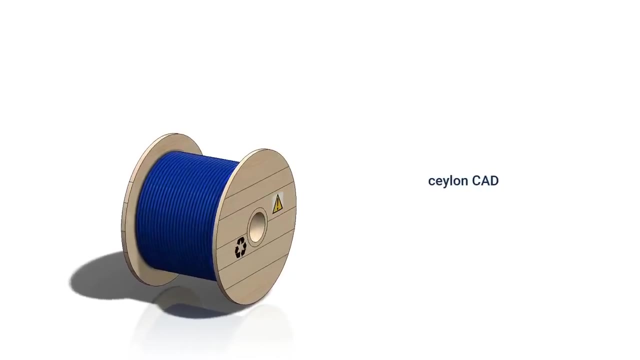 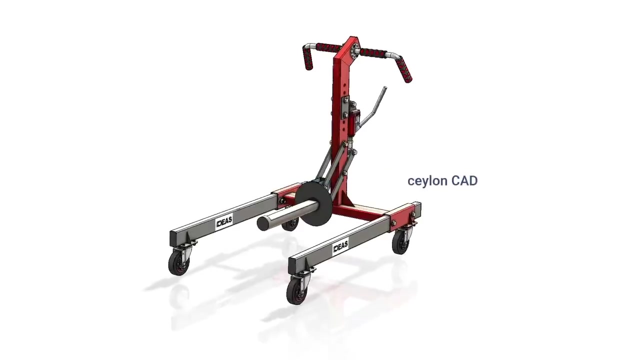 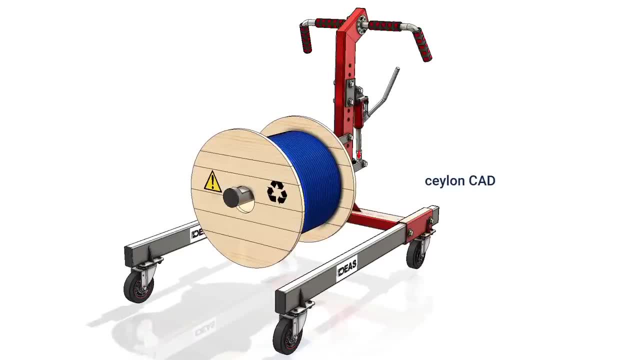 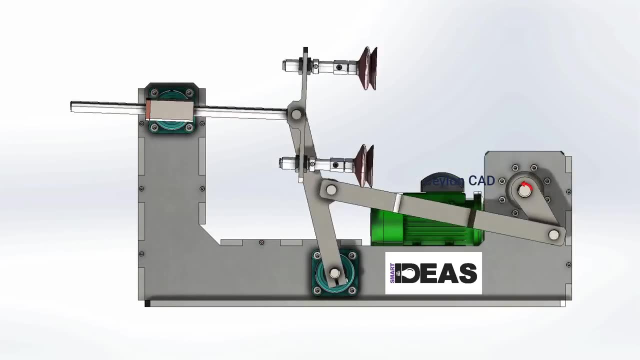 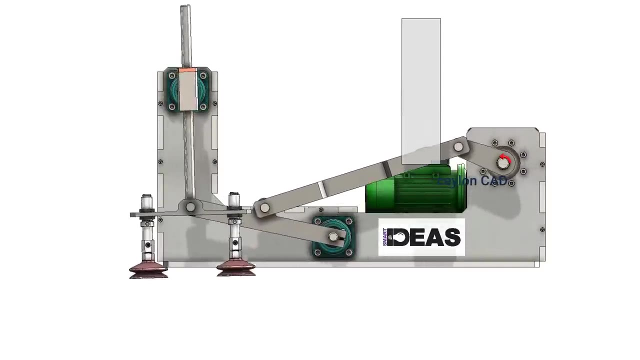 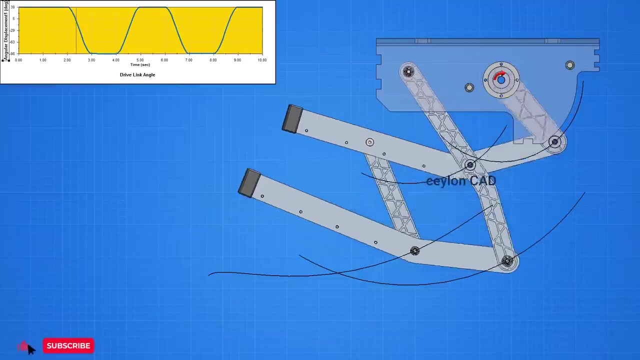 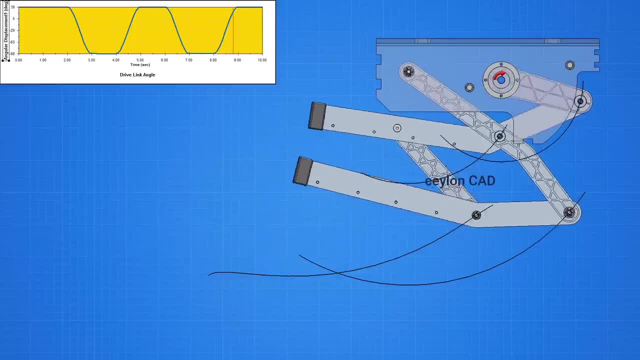 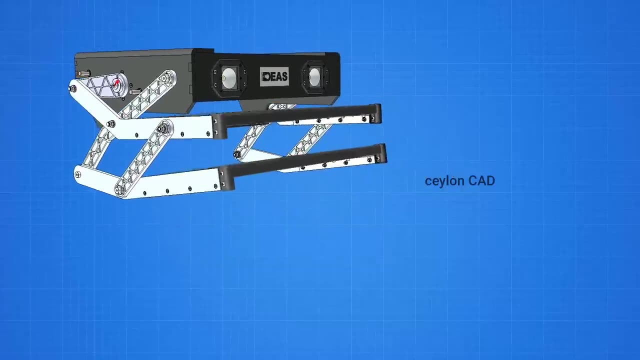 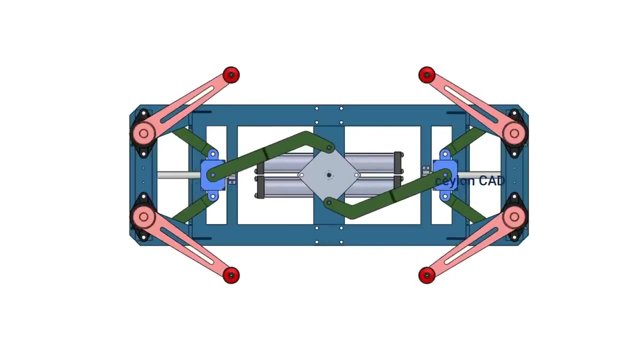 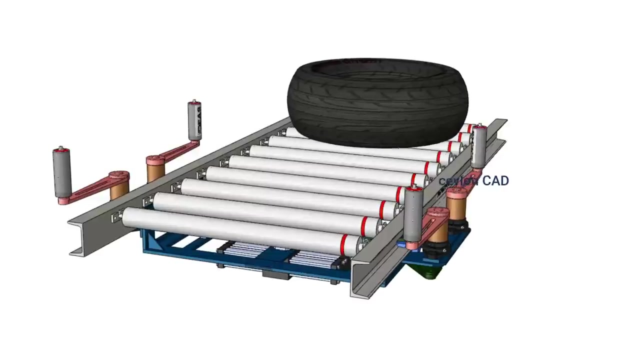 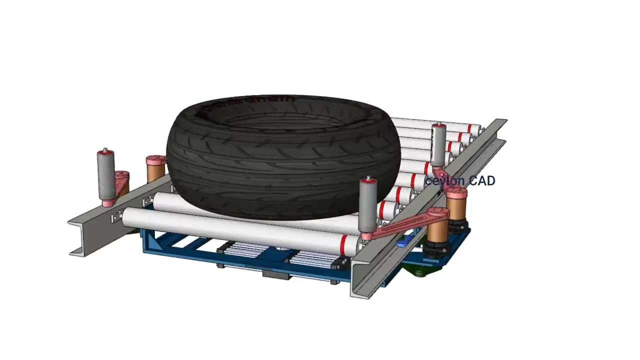 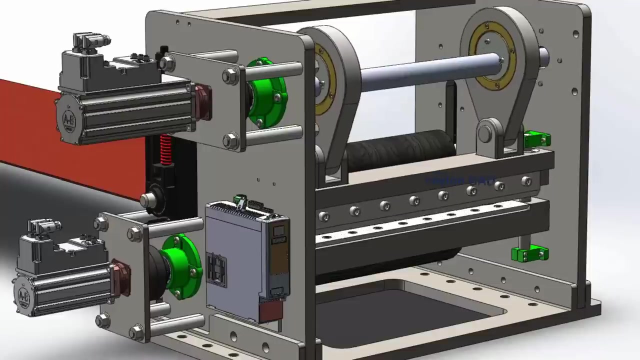 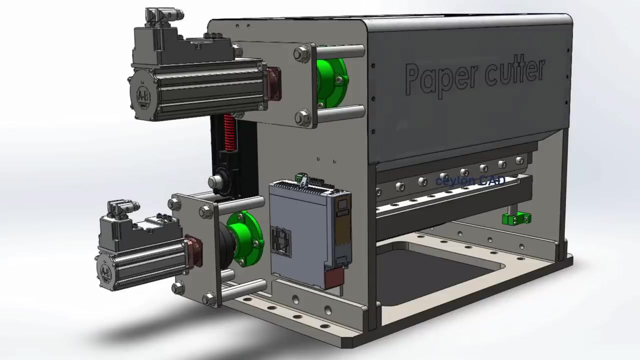 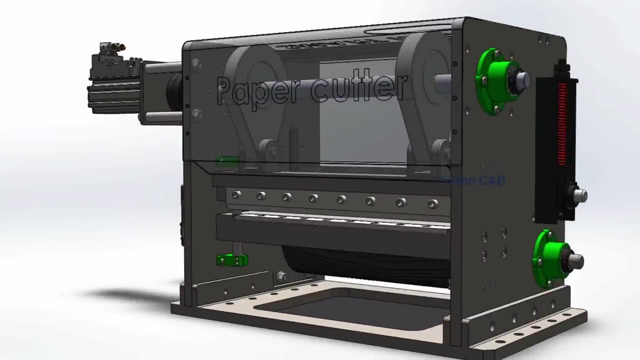 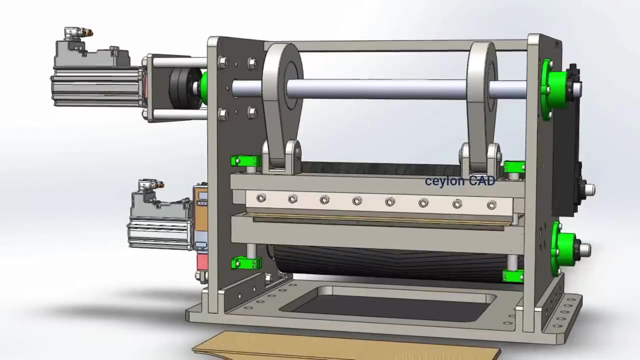 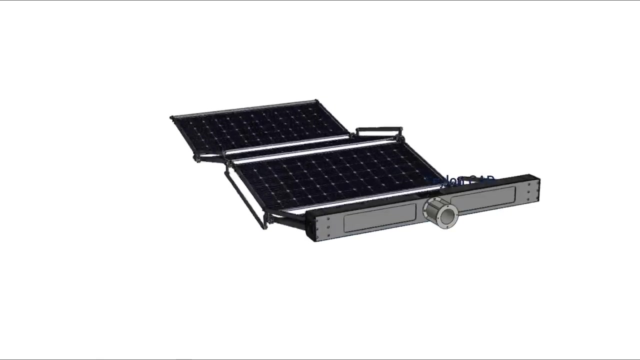 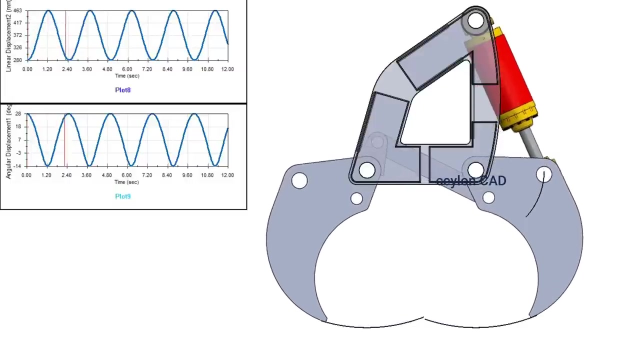 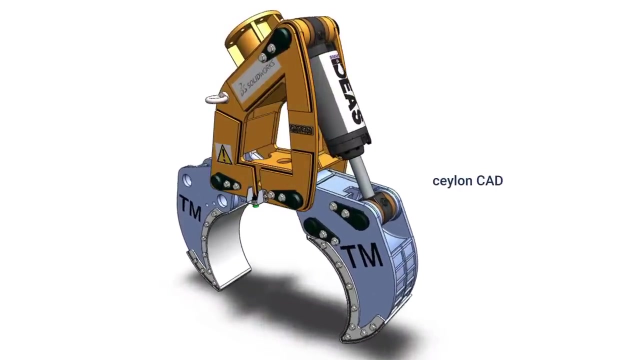 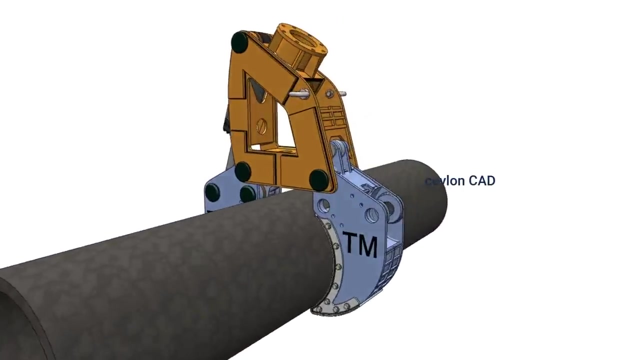 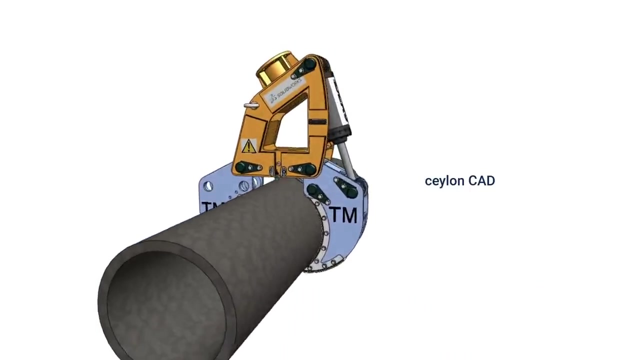 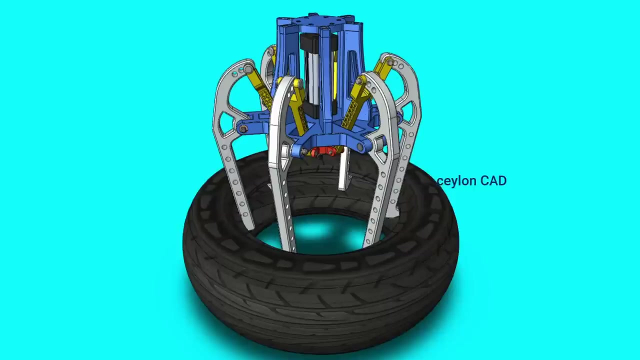 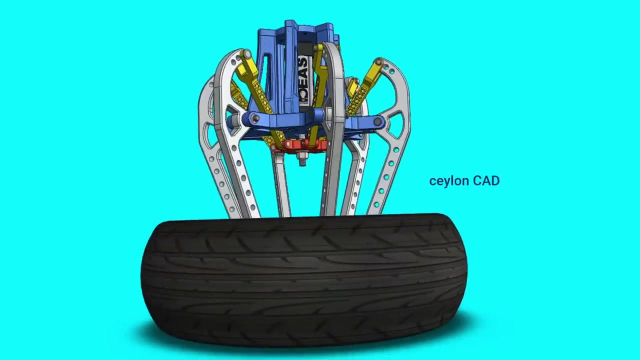 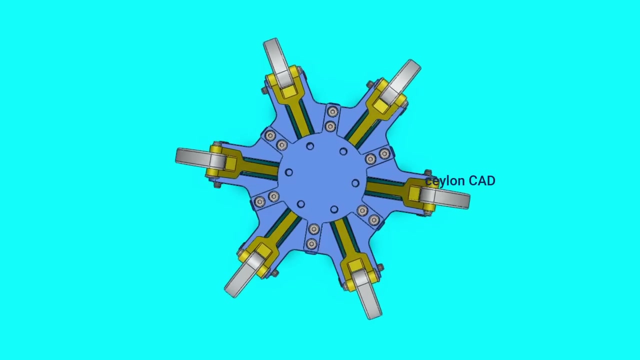 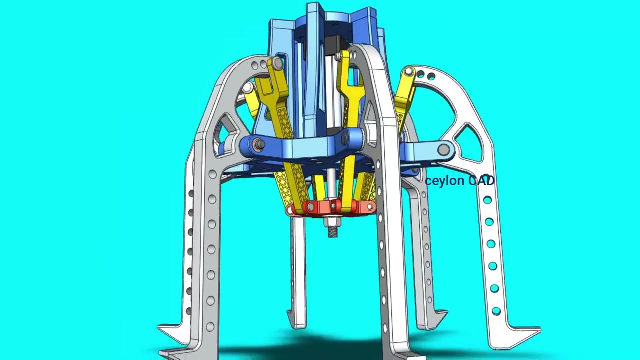 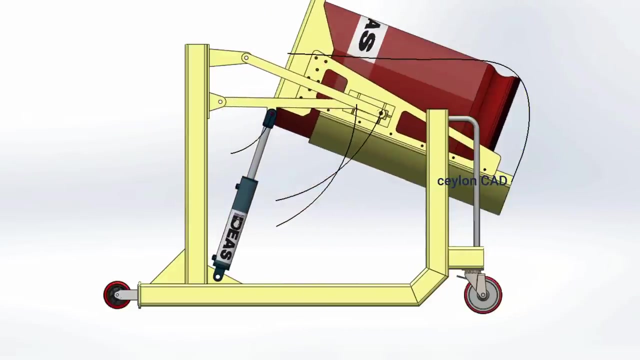 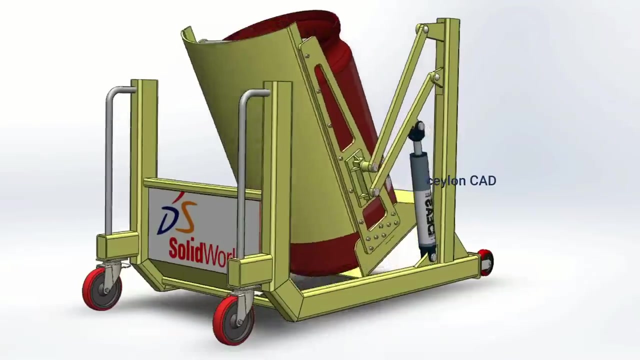 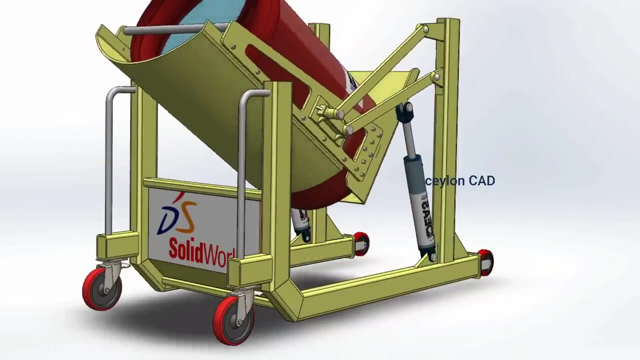 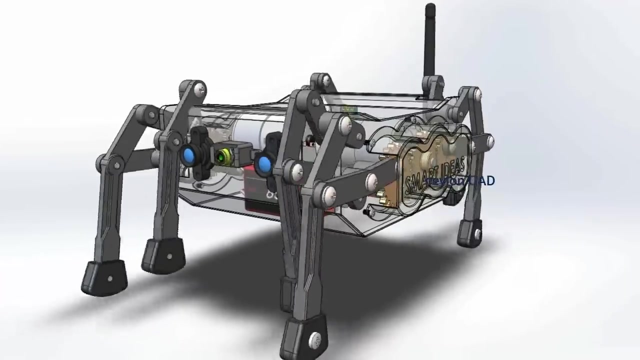 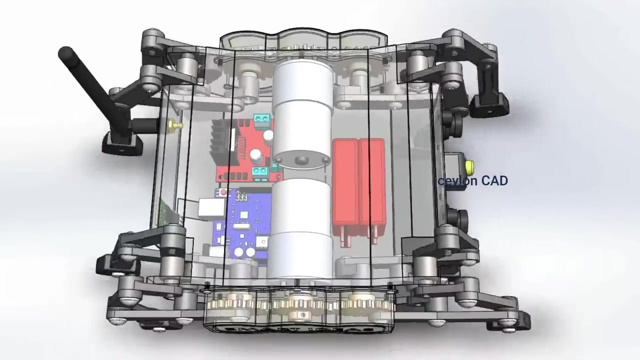 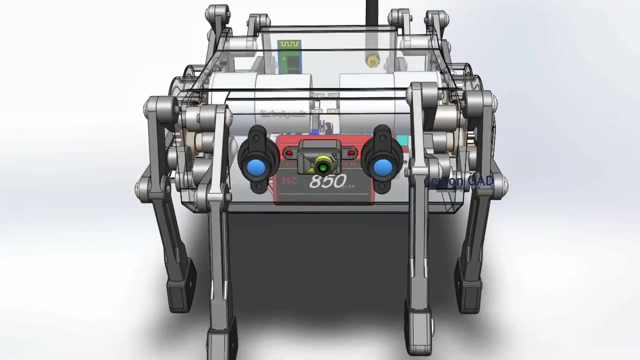 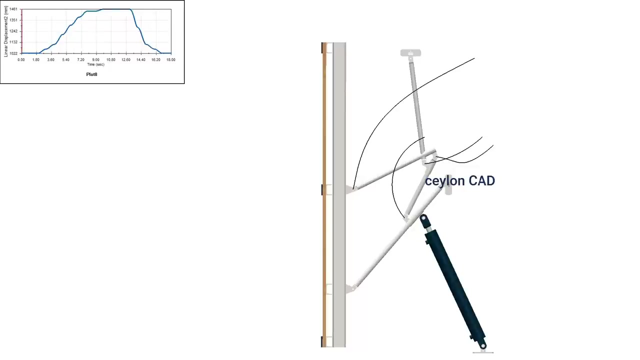 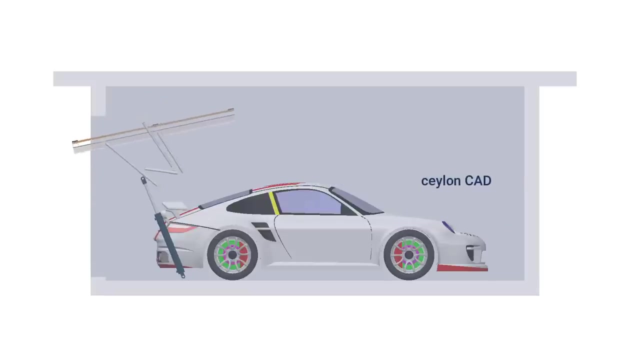 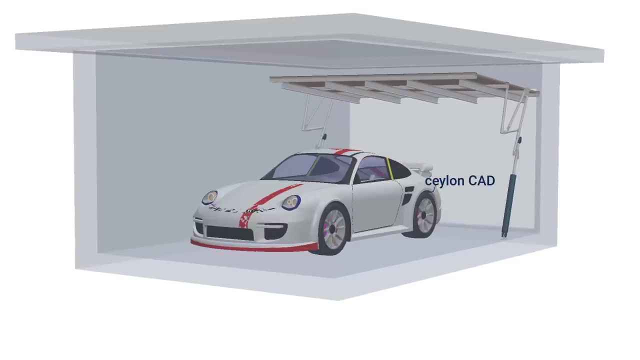 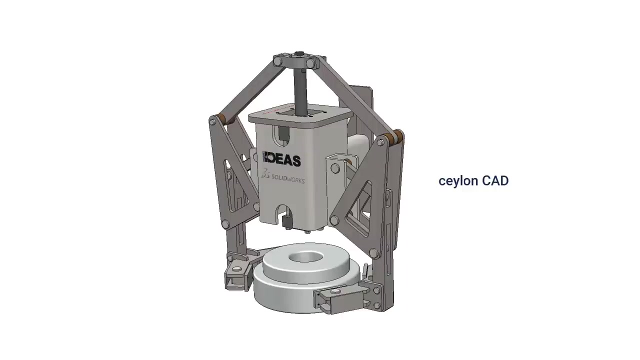 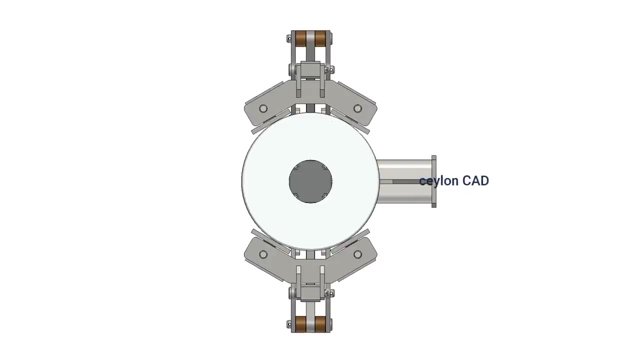 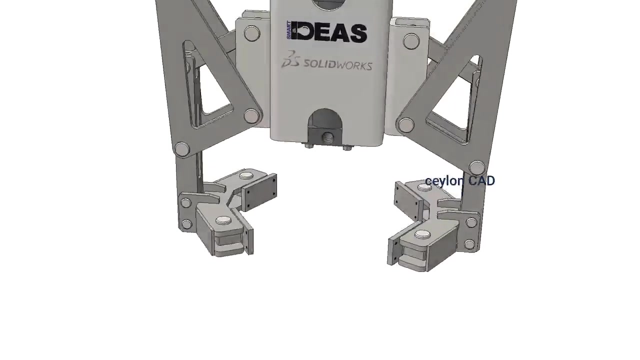 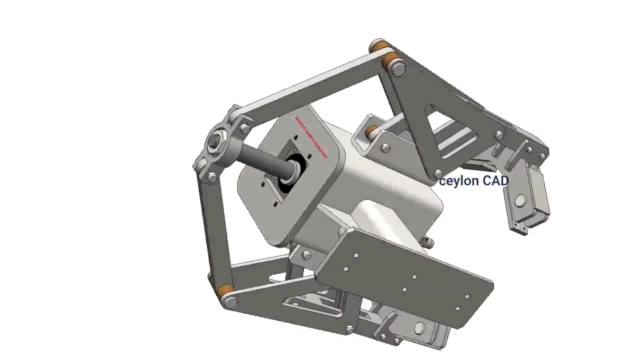